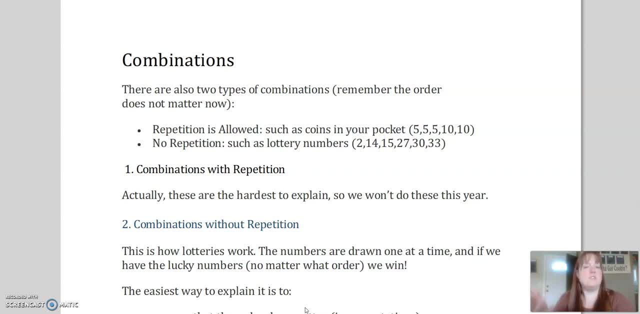 You can't pick someone twice for that. You can't be um in the top three twice. So combinations with repetition we're not actually going to talk about in this um in in this class. That's more for like a full on statistics class that we might talk about it, but not in algebra two. So we're going to talk about combinations without repetition. These are things like lottery winners. So in the lottery it doesn't really matter if you get the numbers in the same order as they pick it out, as long as you get the same numbers right. 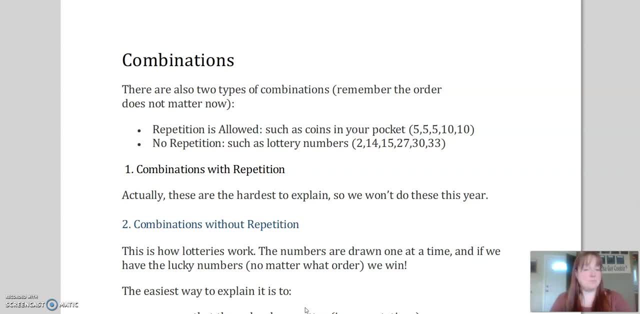 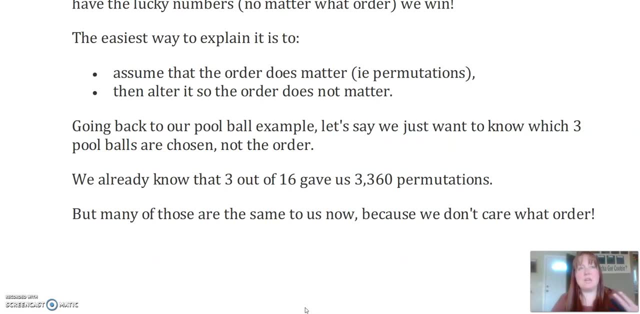 So combinations, not permutations, Because order doesn't matter. So let's, this is the way to explain it, Um, and I hope this doesn't blow your brains too badly, but it's really, um, it's not terrible. So we know how to figure out permutations and we understand the logic behind them. We understand that we use that counting principle to multiply, you know, 10 times, nine times, eight times, seven times six. We understand how to do that. Okay, So basically, with a combination, what we do is we figure out the permutation. 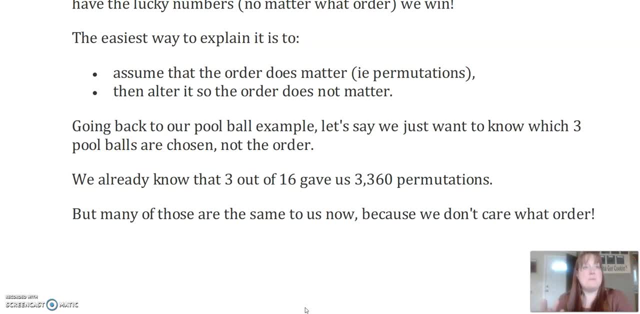 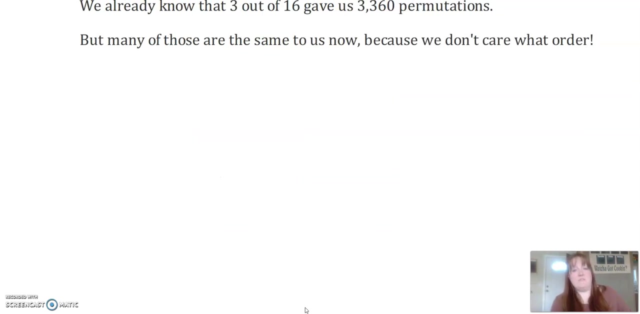 And then we divide it by the number of times we pick it out, And then we divide it by all the different ways that those things that we selected could be ordered. For example, in our pool ball example, um, we had the permutations. There are 3,360 permutations that could be um, that could be formed out of those 16 pool balls. 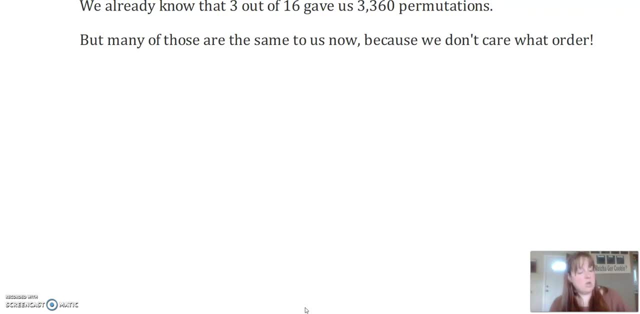 But we know that if we pick out ball number one, two, three in permutations that's different than if we pick out ball two, one, three or three. two, one, those are all different combinations. But in com those are all different permutations In combinations. if I pick out one, two and three, it doesn't matter what order I picked them out in, They're all the same, Okay. 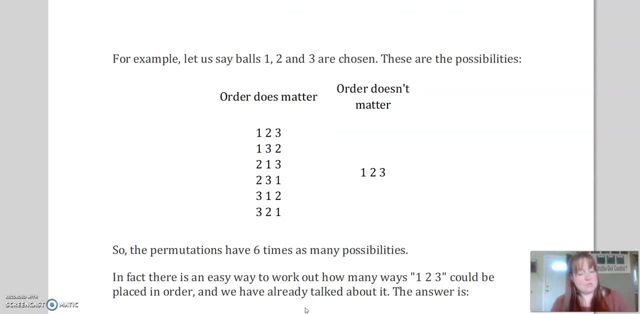 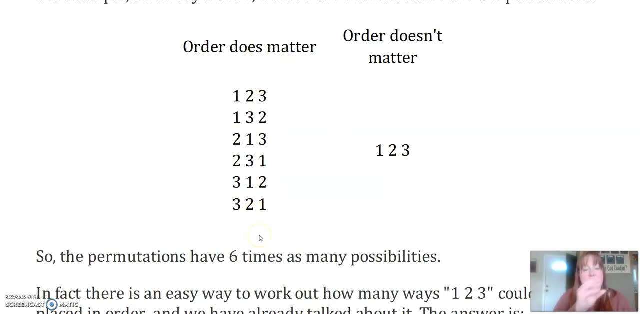 So if I list those with a permutation, there are six different ways that I could pull those three balls out right In in order. But since order doesn't matter, there's only one way that I could combine those right, Because this is like the top three students: It doesn't matter if you're told that you're the top in the top three first, or if you're told last it's, you're still in the top three, right. 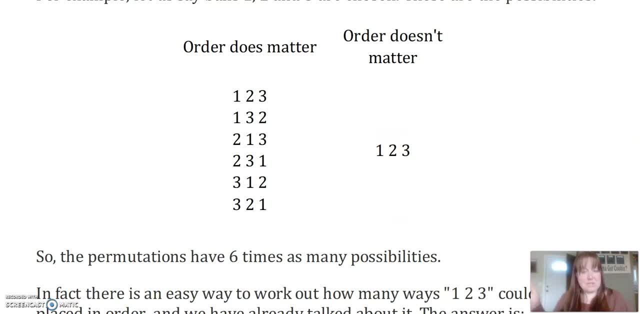 So, basically, what we have to do is we have to take the permutations and we have to divide it by the number of times that we could possibly arrange those numbers that we pulled out. So how many different ways could we arrange the numbers one, two and three? 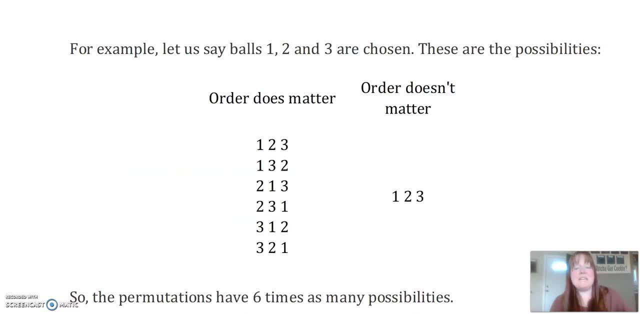 Let's go back to our idea of the fundamental counting principle. Well, the first time I could pick one, I could pick one digit. so that would I would have three options, right. And then the second time I would have two options and the third time I would pick one option. So this would be a permutation with three things. 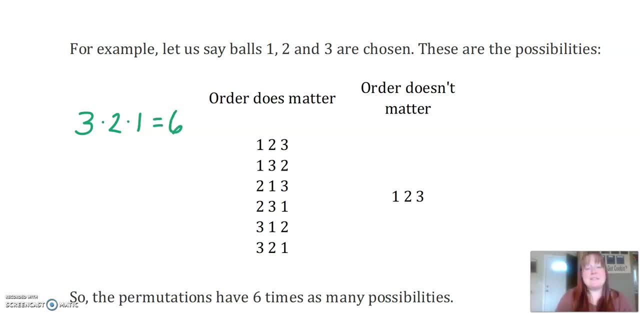 Picking all three of them. So there are six different ways that I could pick that, or three factorial ways. Okay, So we take our permutation, which was 16 factorial divided by 13 factorial, And now we need to divide out all the different ways, all of these extra ways that we could arrange those numbers right. 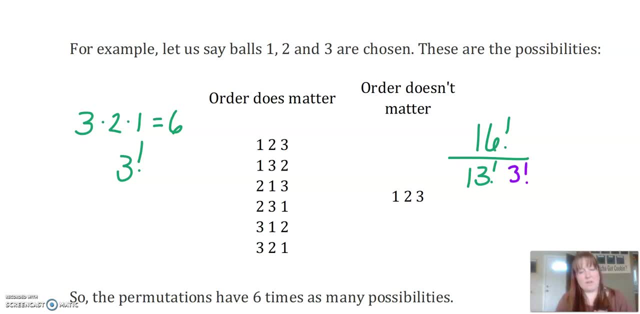 Well, that was three factorial ways. right, There's three factorial. So this is the combinations formula. You'll notice that we have fewer combinations than we need to have permutations, because order doesn't matter. So there's going to be a lot fewer options. 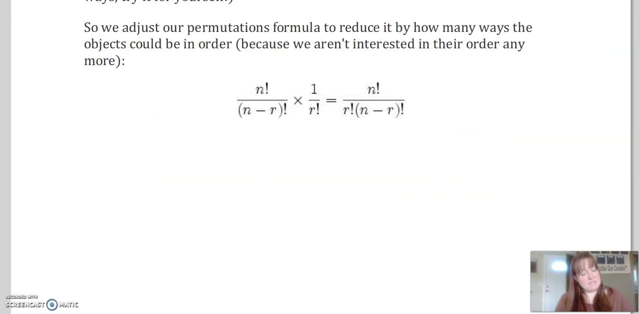 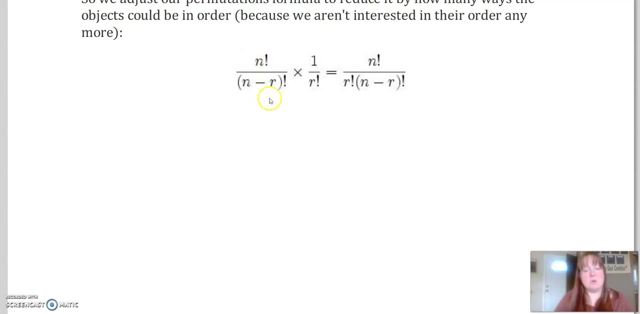 So this is how we would write that. This is our permutations. formula n factorial over n minus r factorial. That's our permutations. And then we divide it by how many ways we can arrange r objects. okay, So we would divide it by r factorial. 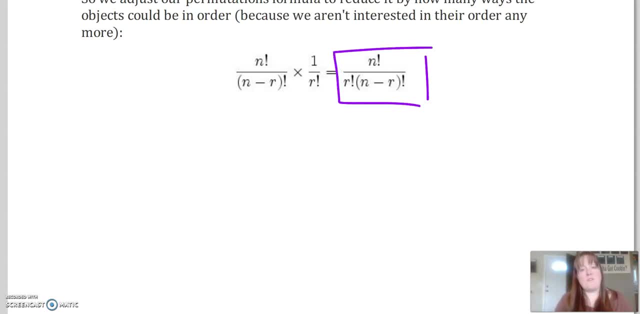 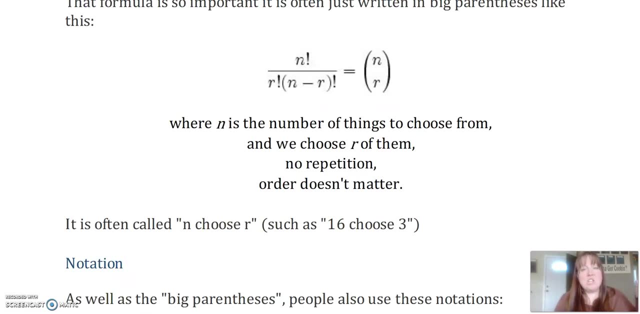 So in the end we end up with n factorial over r factorial times, n minus r factorial. So that's our formula, right there. And combinations are so important and so common that you actually can write them. They have a special notation that you often see, and it's these big parentheses. 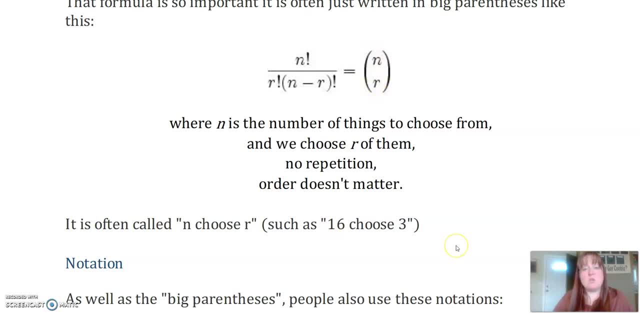 These big parentheses with n on the top and r on the bottom. So remember, n is the number of things we choose from And r is the number of them that we choose. So we actually say n choose r, or 16 choose 3.. 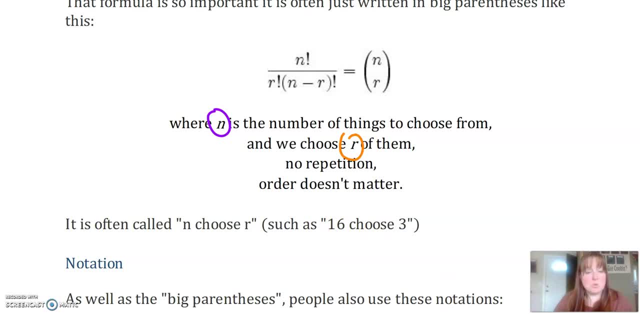 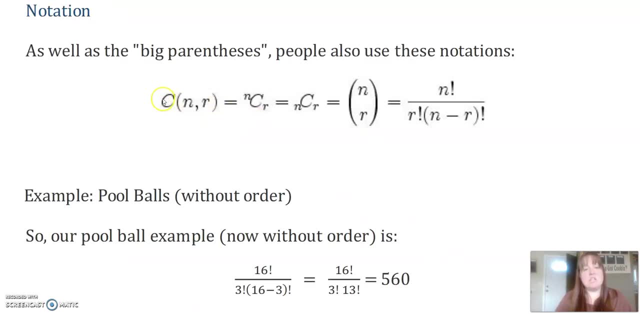 That's actually like a notation that people use in math. So there's some other notations that you might see, Just like in permutations. sometimes you're going to see this notation, But instead of a p it's going to be a c, because we're talking about combinations. 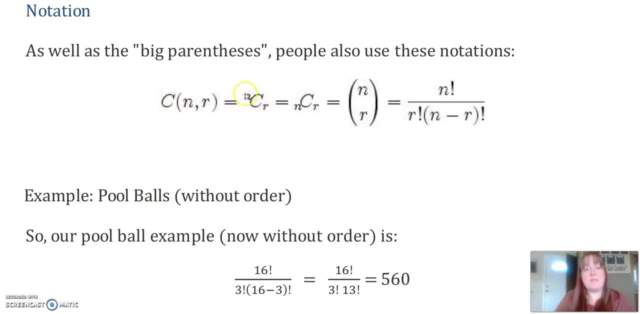 So then you might also see it here with the n and the r On either side of the c. Again, this is the one I see. These two are actually the ones I see most often Where you have the n numbers of things we're picking from. 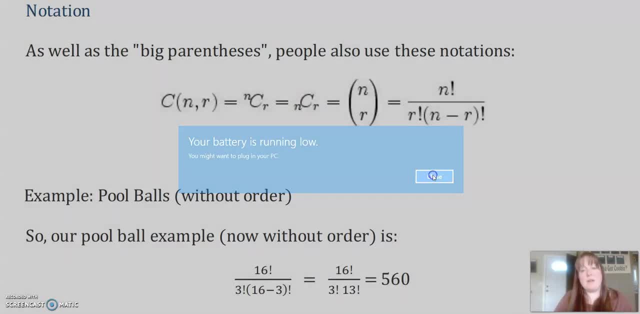 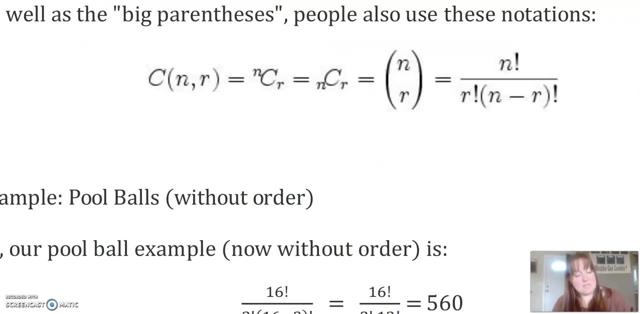 and the r is how many things we pick, Or you're going to see this one. So in the pool ball example you might see it written in any of these ways. You might see c combination: 16, choose 3.. You might see 16, choose 3.. 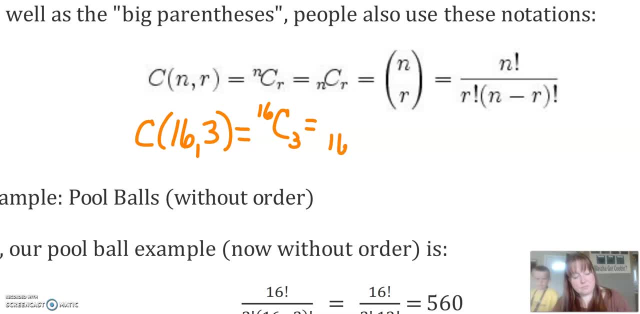 You might see 16 choose 3.. Or you might see 16 choose 3.. These are all different ways to write our pool ball example. Hi, buddy, You know I'm recording a video. Hi, Hang on for just a minute. 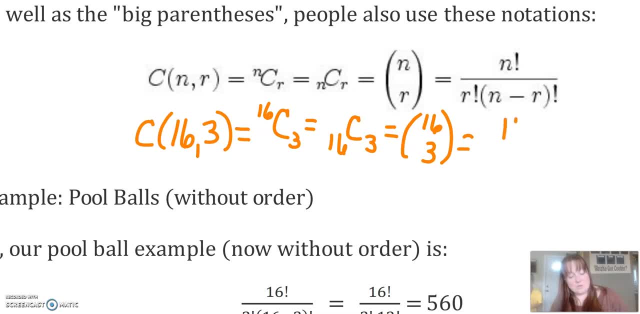 Okay, And then we could do 16 factorial, That would be 16 factorial over 3 factorial, And then n minus r, So that's 16 minus 3, which is 13 factorial. Okay, So we would do it. 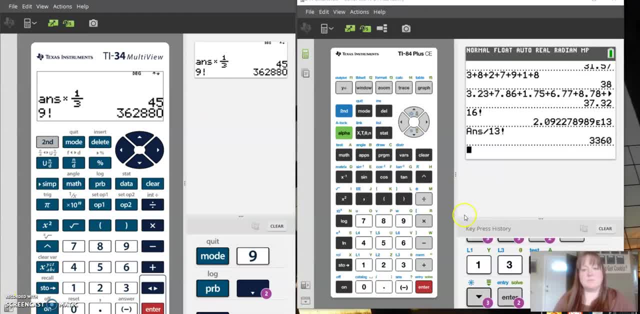 And now let's figure out how to do that in a calculator. I'm going to show you on this calculator. Both calculators work the same. You just need to put the factorial in, Okay. So in this case we had 16 factorial. 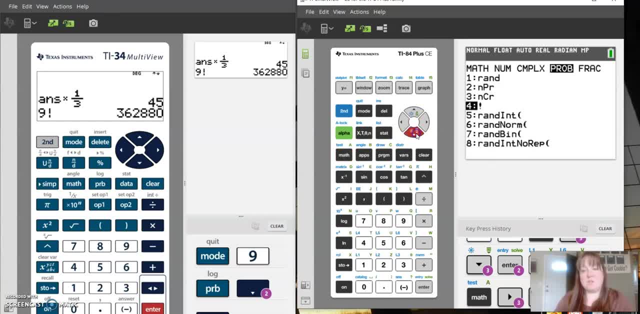 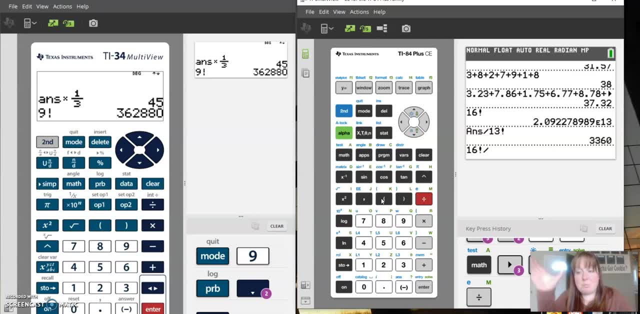 Math. Go over to probability. Go down to factorial Divided by Okay, Now we have 3 factorial times 13 factorial. Remember those are both on the bottom. So remember that our calculator is really actually very good at order of operation. 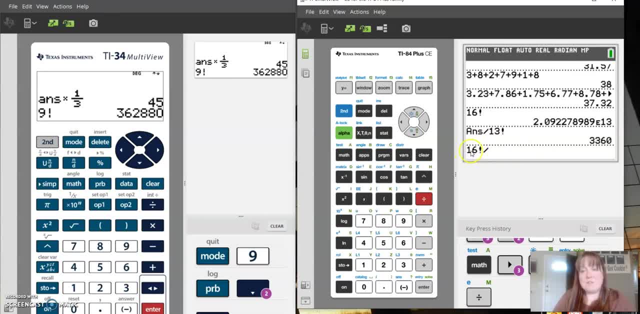 So it's always going to do it in the order that we tell it to do it, And so if we do it this way, it's actually going to do the division first before it does the multiplication on the bottom. So we need to put parentheses around that. 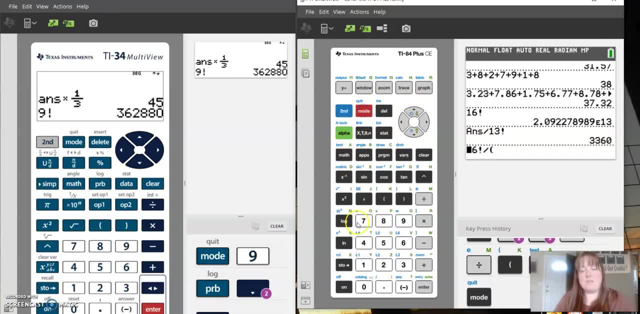 And then we can do math. Nope, Don't do math yet We got to do 3 factorial, 3 factorial Times, 13 factorial, And then we close those parentheses. So this says to our calculator: do this on the bottom first, before you do the division. 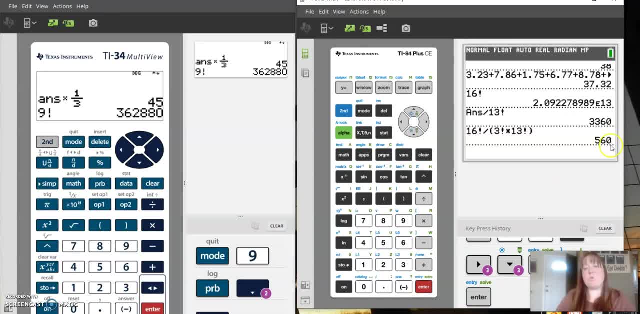 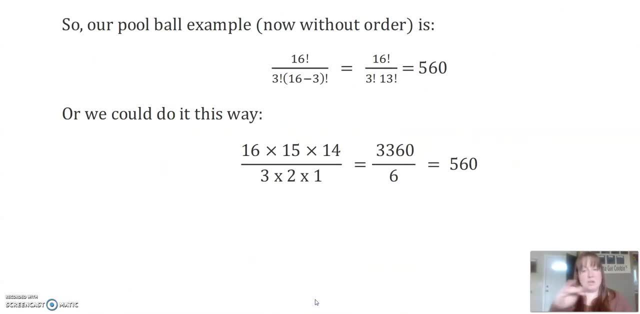 We push enter And we're going to get 560.. So there were 3,360 different permutations for this option, But there's only 560 different ways we could order them. if order doesn't matter, Okay, So if we do it that way, we can put it in our calculator that way. 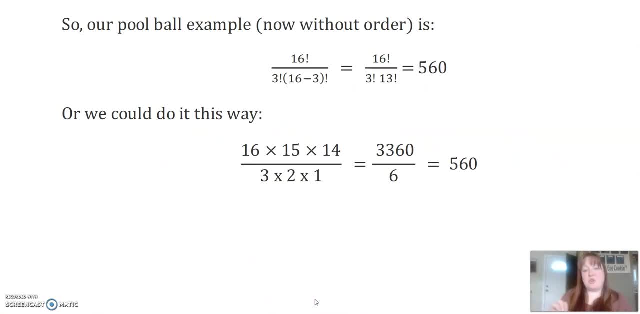 Or you could do a little bit of algebra first and then just not have to deal with factorial, Because remember 16 factorial divided by 13 factorial, it canceled out that 13 times 12 times 11 times 10.. So 16 factorial divided by 13 factorial is just 16 times 15 times 14.. 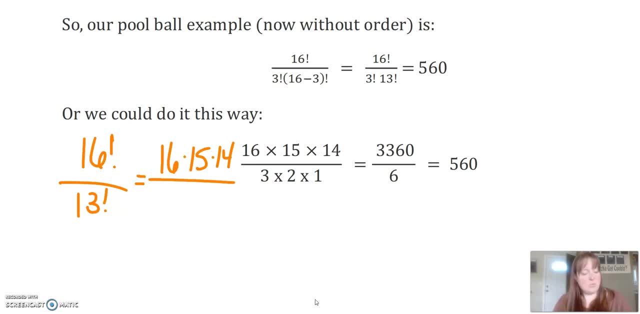 Okay, So you could write it like that. And then: what is 3 factorial, 3 factorial? Well, that's 3 times 2 times 1.. So we could do that math and then do it again, and we'd get 560.. 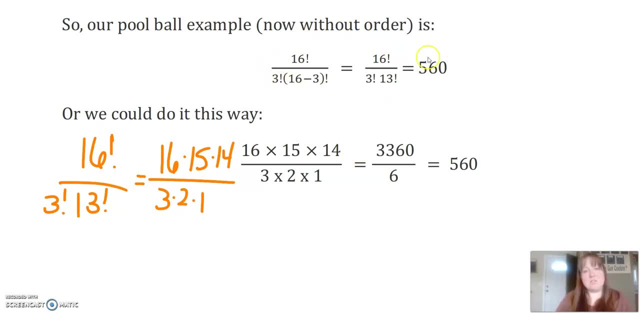 Either way works. Honestly, this is an easier, cleaner way once you get used to it, But this feels more natural at first. 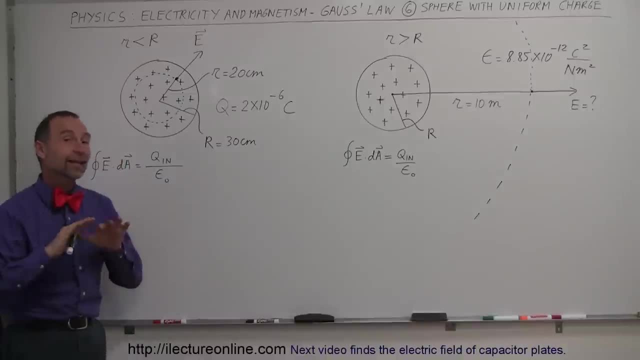 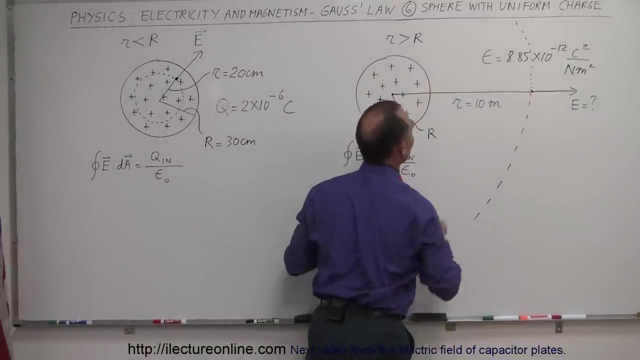 Welcome to ElectronLine. and here we're going to use Gauss's law and the Gaussian surface to find the electric field inside a spherical object that has charge throughout the entire object, and here we're going to find the electric field strength outside that very same object. So here what's? 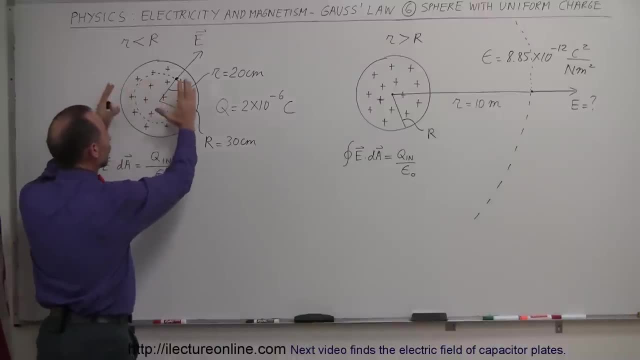 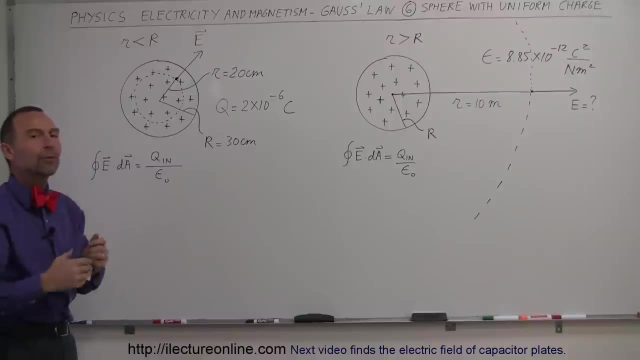 different is that we don't have a conductor with charge on the surface. here. we have an object with surface all throughout the sphere. so these are spherical shaped objects with charge equally distributed everywhere inside the sphere and we want to know the electric field strength. let's say: